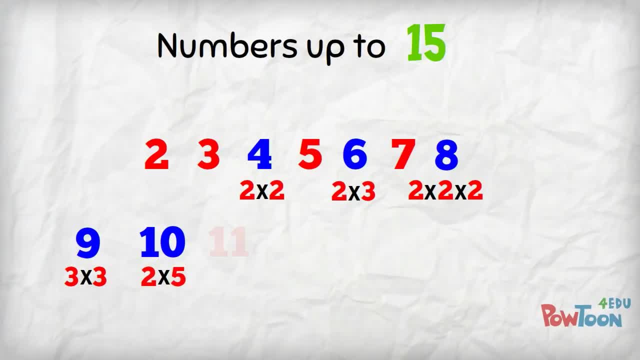 We get 10 from 2 times 5, 11 is prime, 12 is from 2 times 2 times 3, 13 is prime, 14 is from 2 times 7 and we get 15 from 3 times 5. Prime factorization means: 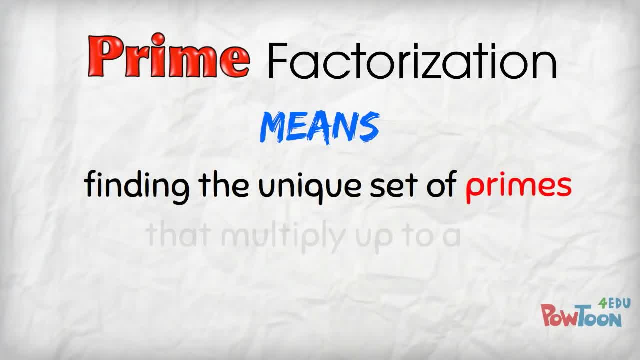 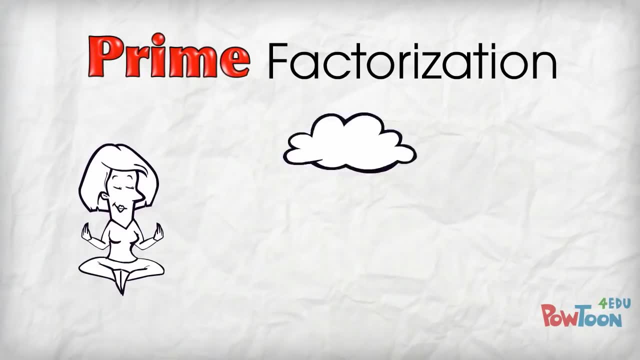 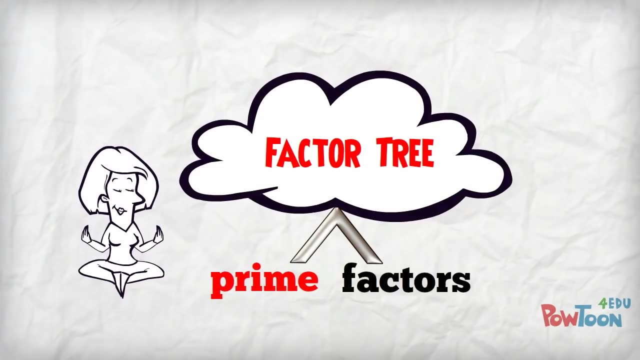 finding that single set of prime numbers that multiply up to a given composite number. To do a prime factorization, we can use a factor tree to help us split each composite number apart into its prime factors. Let's do an example: 18 We split 18 into factors. 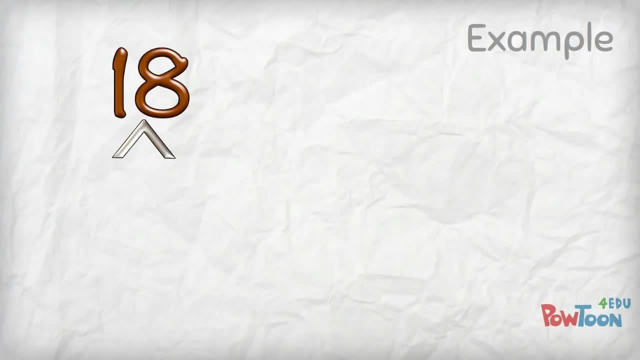 until we can't split any more. I am using red for prime numbers and blue for composite numbers. I say to myself: 18 comes from 2 times 9. I circle 2 as a prime number. I will come back to it later. 9 is a composite number. 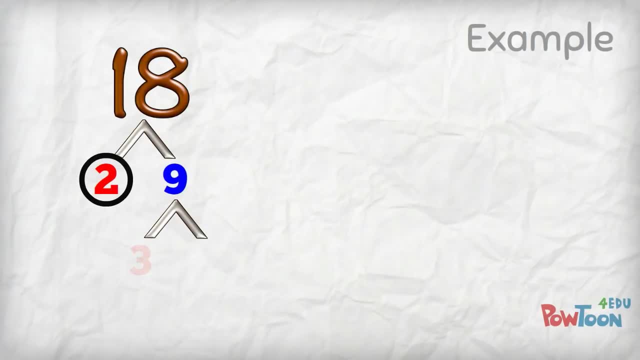 so I split it down, I get 9 from 3 times 3. 3 is a prime number, so I circle both of them too. I have no composite numbers left. so now I know I have found all the prime factors Next to the factor tree. 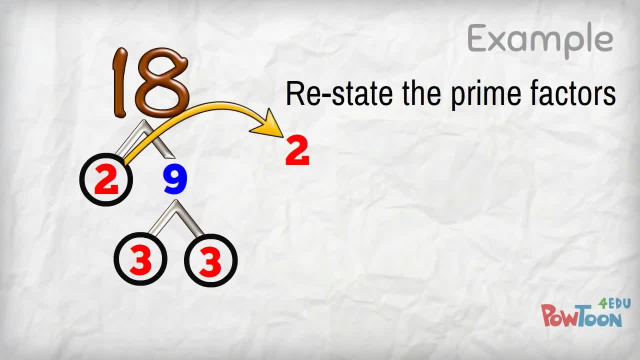 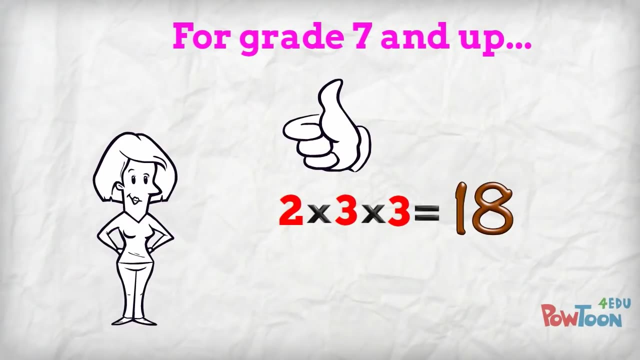 I restate the prime factors: 2 times 3 times 3 is 18. It's correct, but it's not quite finished. To do a really great job on prime factorization, we show a factor that is repeated by using exponents. We call it. 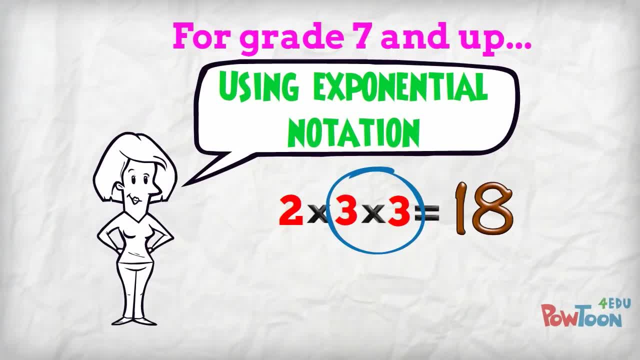 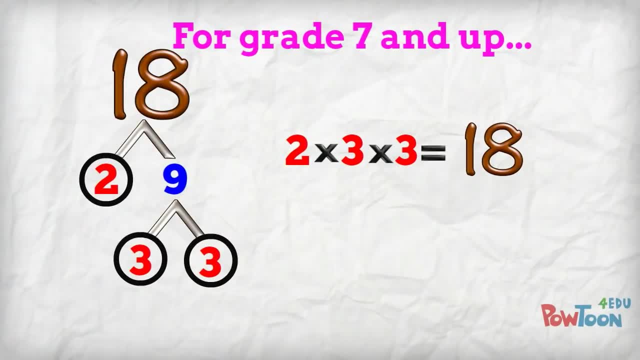 using exponential notation. It sounds fancy but it's easy enough. Check it out. How many 3's have I got? 2. So I say 2 times 3 to the power. 2, because 3 is used twice, is 18. It makes the final answer very tidy.